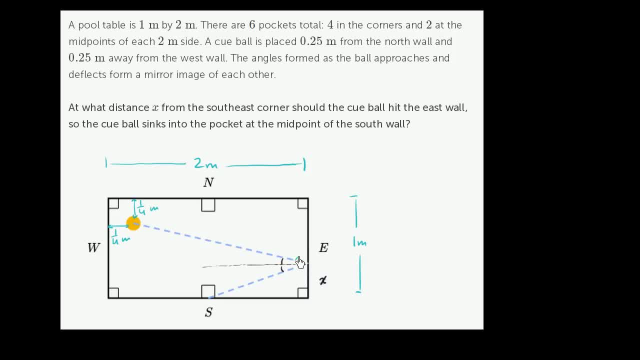 If those two angles are congruent, then this angle, which is just that black angle, which is complementary to that black angle, must be equal to this angle. Each of these are going to be 90 degrees minus that black angle right over there. 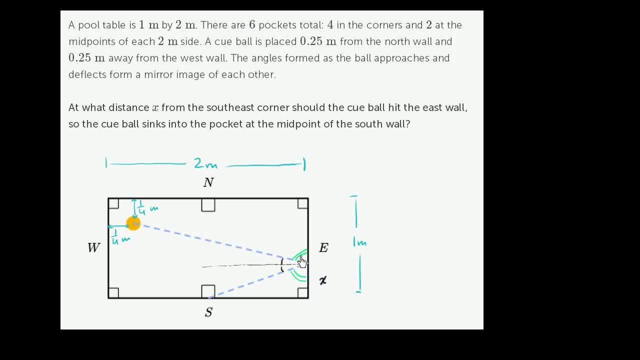 So you have, this angle is congruent to that angle, And now we can construct two right triangles. So you can imagine one up here. This is the larger one, So you could kind of imagine this is our approach: right triangle right over here. 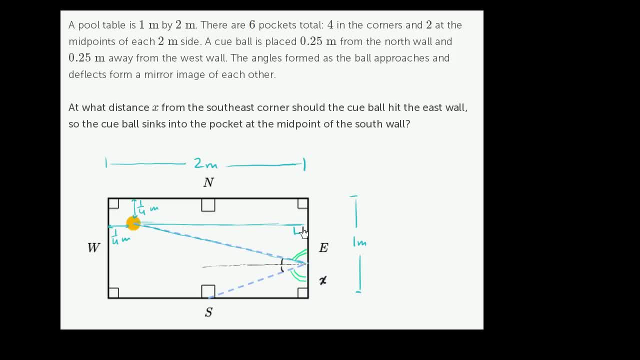 So the top of it is parallel to the side of the pool table And then this is our deflection right triangle right over here, And the whole reason why I show that these two green angles are going to be congruent is to show that these two triangles are. 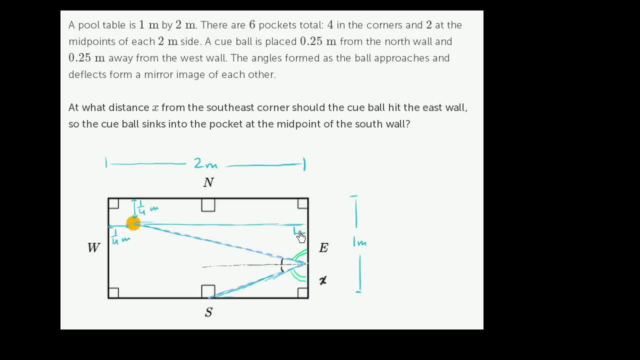 similar to each other. How do we know they're similar? Well, if you have two angles. they both have a 90 degree angle And they both have this green angle. So that means that the third angle must also be the same. 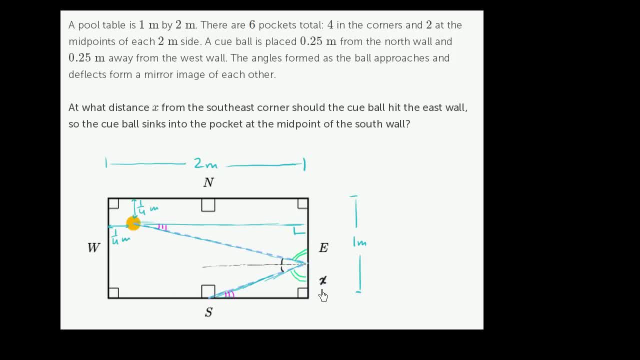 If you know two angles, you know what the third angle has to be. If two corresponding angles of two different triangles are congruent, then the triangles are going to be similar. So this top triangle is similar to this bottom triangle, And what that helps us is that means. 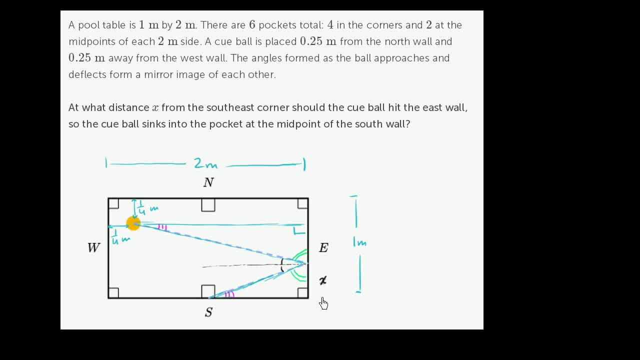 that the ratio of corresponding parts of the triangle, the lengths of the ratio of the lengths of corresponding parts of those triangles, are going to be the same. So, for example, we've already said that this distance, Let's figure out what we know about these triangles. 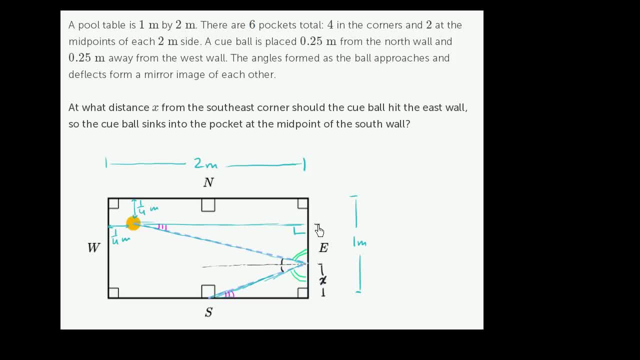 So that distance is at is x. Now, what is this distance right over here? What is this distance right over here going to be? Well, let's think about it a little bit. We know that this distance is 1 fourth of a meter. 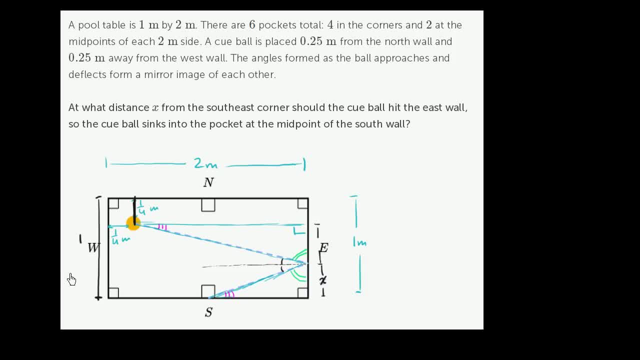 We know that this entire distance is 1 meter. So this distance- right, let me do this in a color, you can see this distance right over here- is going to be 3 fourths of a meter. And so if this whole thing, if this distance, 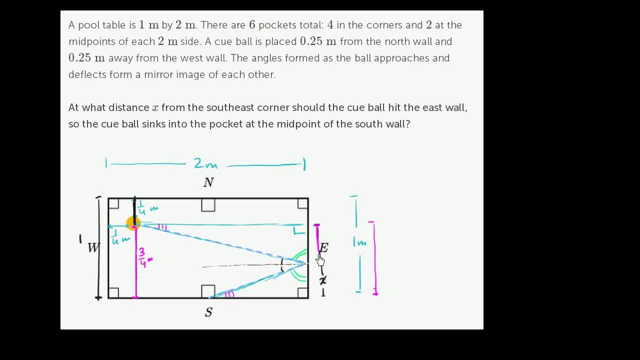 is 3 fourths of a meter, then this part right over here is going to be 3 fourths minus x meters. So let me write that down: 3 fourths minus x is this magenta length, And what else do we know? 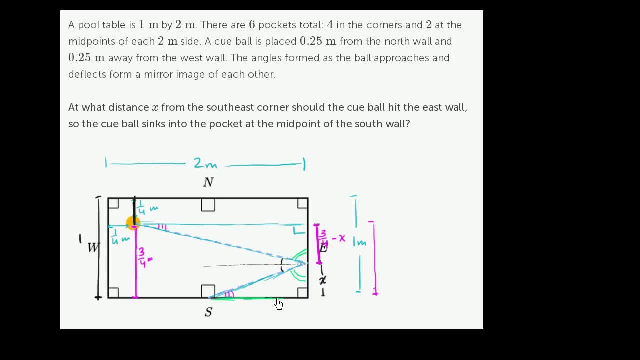 Well, we definitely know the length of this segment right over here. We know that the pockets are 1 meter apart, So that is 1 meter, And we also know the length of this segment. We know that this is 1 meter and that this is another 3. 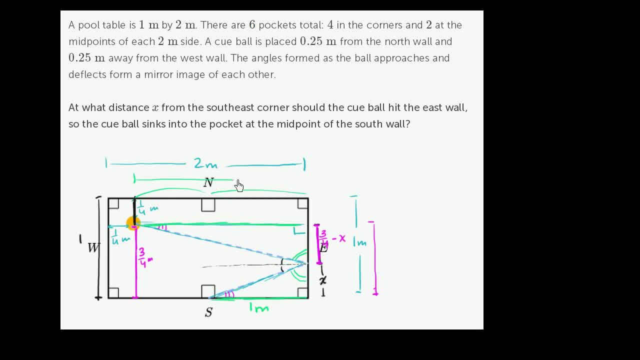 fourths of a meter. So this whole distance right over here is 1 and 3 fourths meters, or we could write that as 7 fourths meters. So let me write it like this: This is 7 fourths. I like to write everything as an improper fraction. 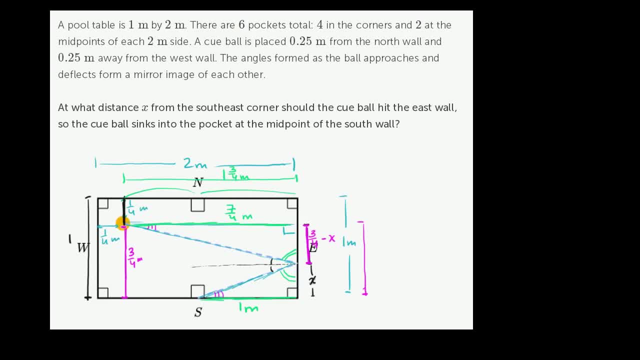 because I have a feeling that I'm going to have to do some ratios in a second. So corresponding parts of these triangles, these two triangles are similar, so corresponding parts are going to have the same ratio. So, for example, this green segment right over here: 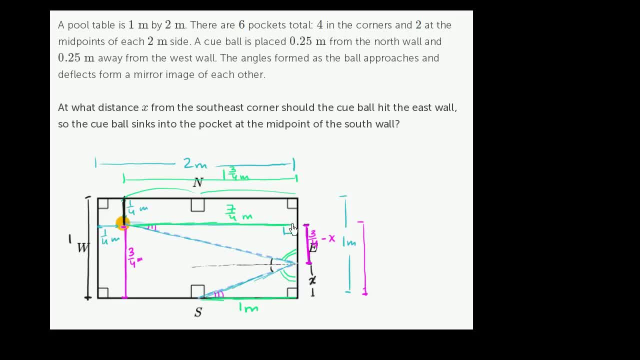 this is the longer side. that's not the hypotenuse of this top right triangle. That's going to correspond to the longer side. that's not the hypotenuse of this triangle, The sides that are opposite this green angle. they correspond to each other. 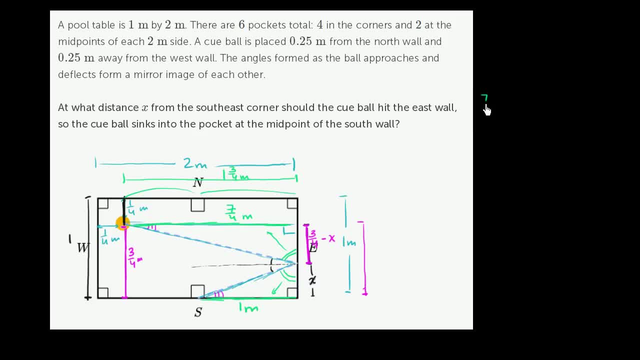 So we could say that the ratio of 7 fourths to 1, the ratio of 7 fourths meters to 1 meter is going to be equal to the ratio of the sides that are opposite the magenta angles. So it's going to be equal to 3 fourths minus x to x. 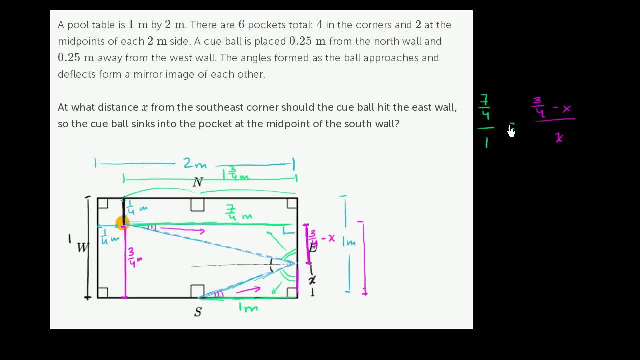 I'm just showing that the ratio of corresponding parts are the same. So let's now just solve for x. So let's see, if we multiply both sides of this by x on the left-hand side, we end up with 7 fourths x. 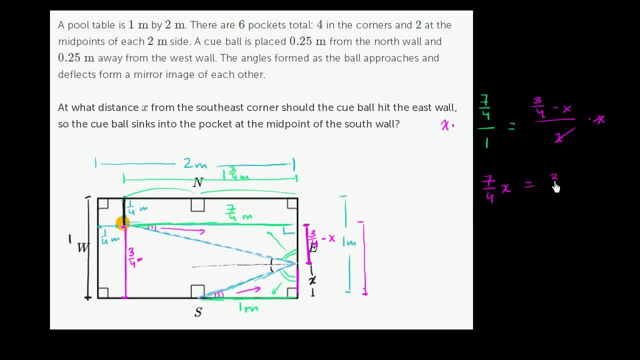 And on the right-hand side, we're left with 3 fourths minus x. Well, now we can add an x to both sides And we're going to get 7 fourths x plus another 4 fourths. x is going to give us 11 fourths. x is equal to 3 fourths.